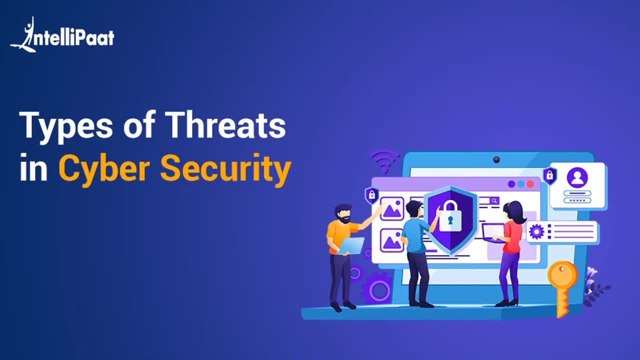 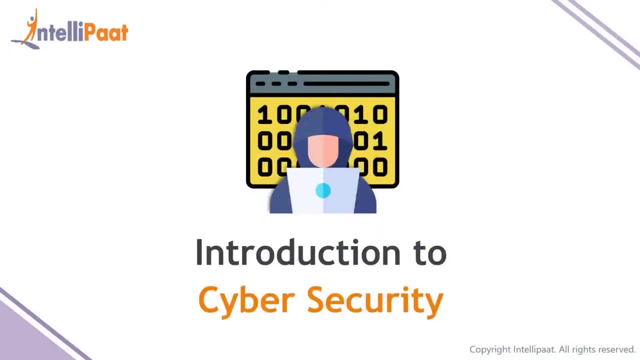 of threats in cybersecurity. but before we actually begin, be sure to hit that subscribe button and click on that bell notification icon so you don't miss out on any updates from us. so, without any further ado, let us begin. so, firstly, we have introduction to cyber security. now this is a 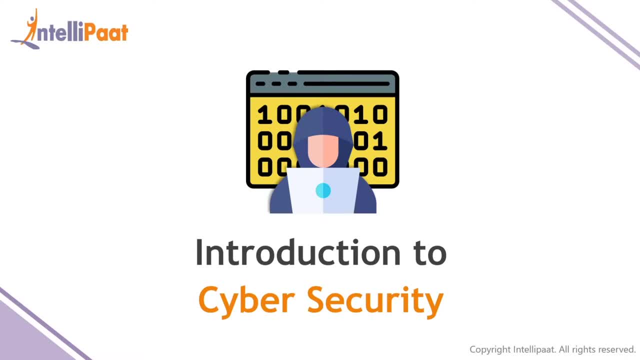 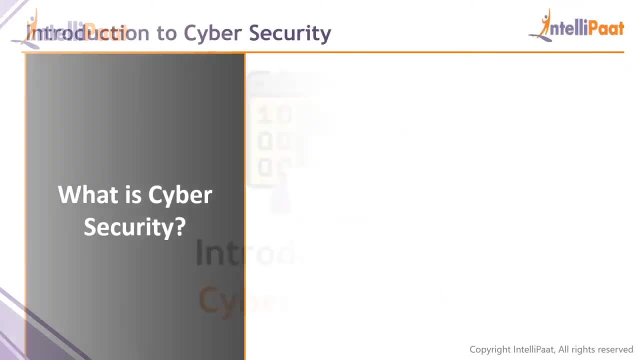 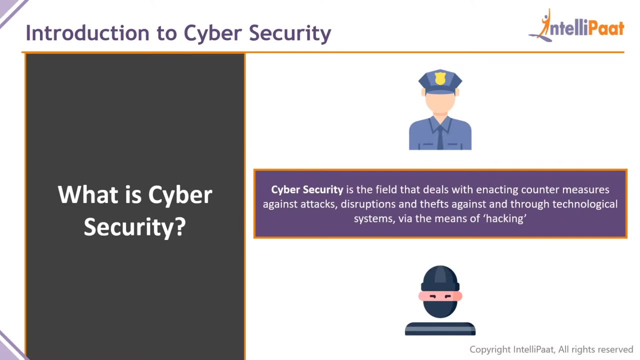 very important aspect to dwell into before we actually get to the threats in cyber security, or the cyber threats as we like to call them. so the first question that comes up is: what is cyber security? now, cyber security is theoretically defined as the field that deals with enacting 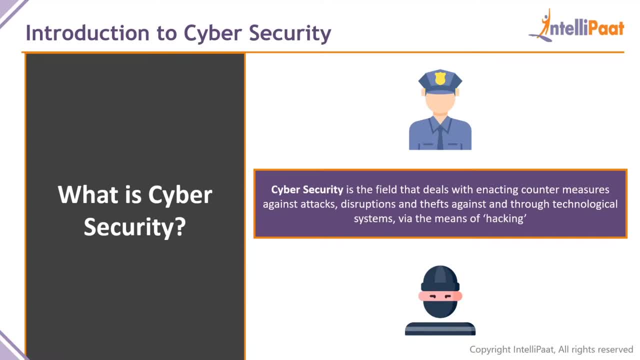 counter measures against attacks, disruptions and thefts against and through technological systems via the means of hacking. so what this tells us is that there is a process which is termed as hacking, and this can be used to attack, disrupt or basically steal anybody's data, money or information. so what is this process all about? 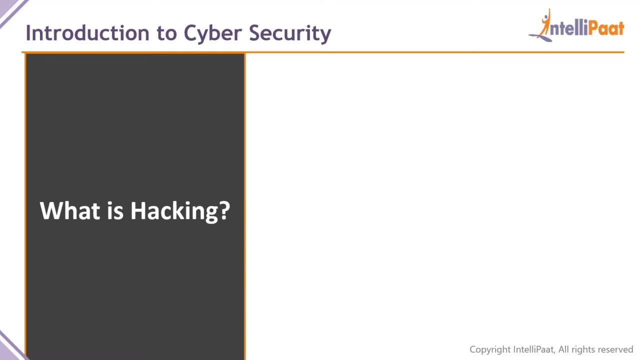 what is hacking? so let us understand what hacking is in the first place. hacking- theoretically it is defined as gaining unauthorized access to a computer system or a network. so any system that you don't have original access to, then you don't have authorization to if you use some underhanded. 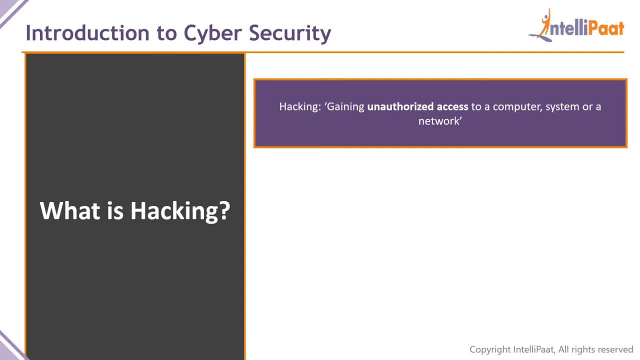 means to gain access to that system. you are not going to get access to that system. you are going to get access to that system. you are essentially hacking that system. so, uh, you, if you're a hacker and there is a secure, secure system that you need to hack, there are obviously security measures. 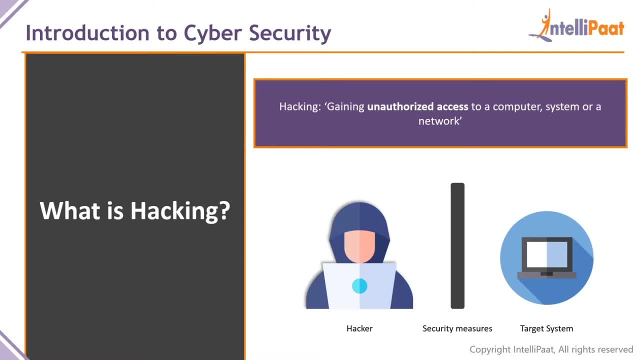 that are put into place between you and the target system. so there are two ways in which you can hack that target system. firstly, you can bypass those security measures by applying some loophole, or you can crack those security measures. so these are essentially the two ways, the gist of the two ways in which hacking happens in the real world as well. so 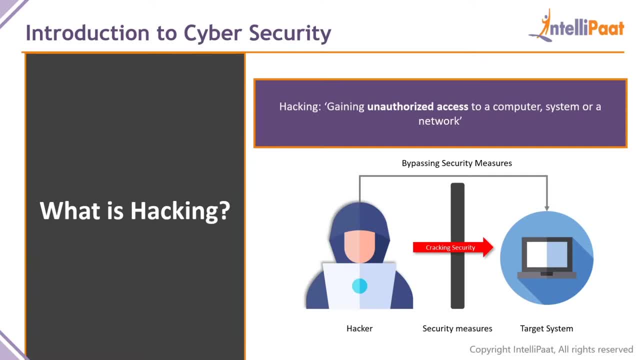 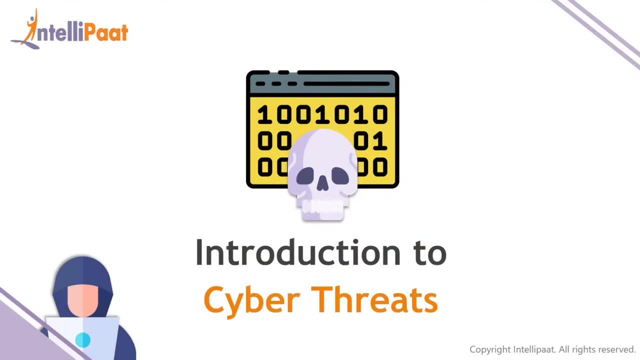 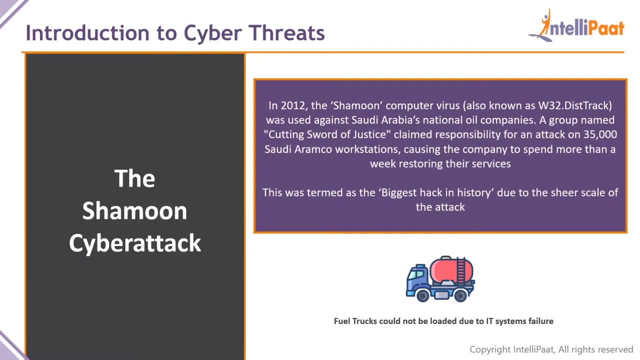 now that we understand what hacking is, now that we understand what the study of cyber security is all about, let us get into the threats in cyber security, or the cyber threats, so the introduction to cyber threats. so firstly, let us understand a little bit of background information first, 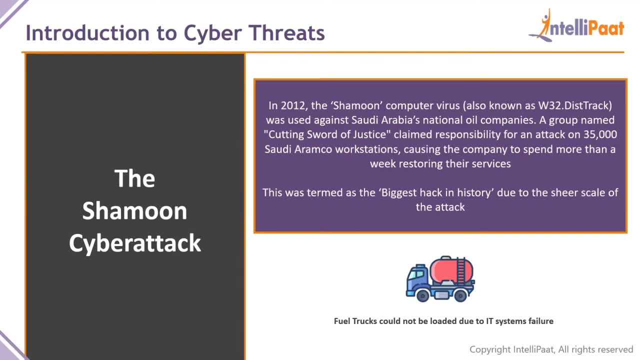 so there was this attack, which was termed as the biggest hack in history. it was called the shamoon cyber attack. so essentially, what happened was that, in 2012, a group known as the cutting sword of justice claimed responsibility for the attack, which was the shamoon computer virus attack, also known as the w32 dist track attack because it affected 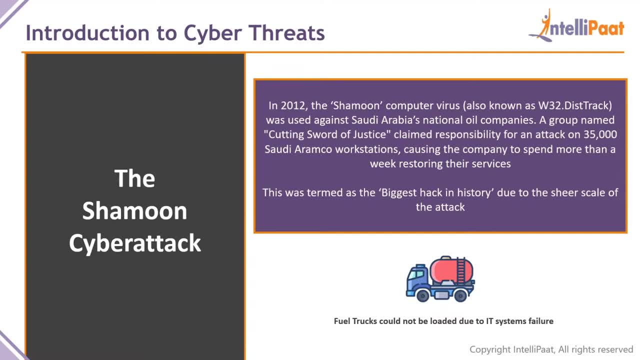 windows net32 bit systems. right so these operating systems were being used in the workstations of saudi arabia's national oil companies for their transactional activity. right so what this virus did was it affected 35 000 workstations of a company known as saudi aramco, which is an oil 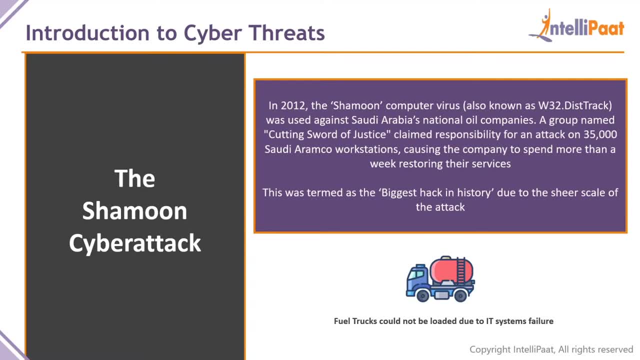 company in saudi arabia. so what this did was it caused the business to shut down for a week until their services were restored back to normal. this shutdown happened because every transactional activity that was happening was happening through these workstations, and when these workstations 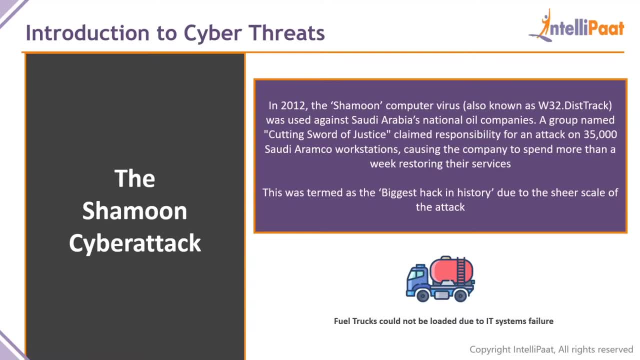 stopped working. essentially, the business shut down because no transactional activity could happen. the fuel trucks which were supposed to carry the oil could not be filled up because the documentation and the records could not be maintained of it and, as we can imagine, oil is an expensive commodity and due to the entire operation, shutting down for a week, how much loss. 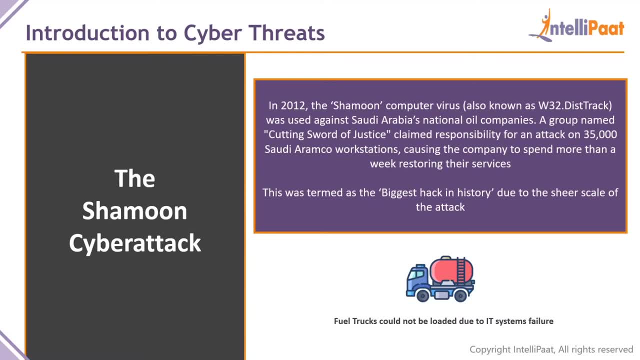 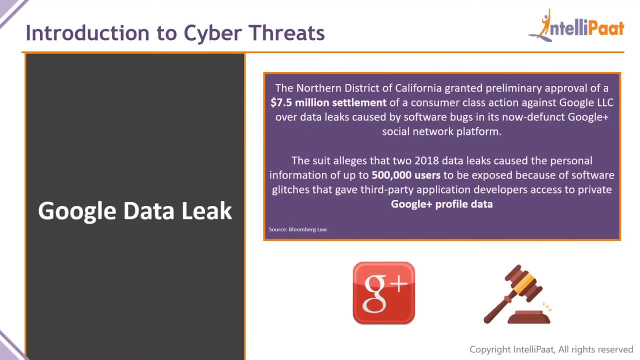 it could have caused. so because of the sheer scale of this attack and the monetary loss, because of the fact it was termed as the biggest hack in history, and there's another example that we can take up of cyber attacks. so the this is not exactly a cyber attack, as much as it is a negligence on the. 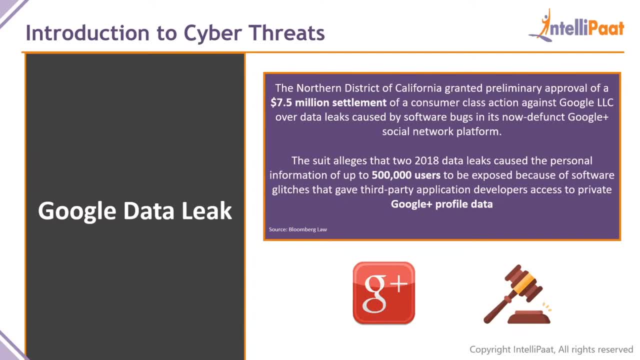 part of google. so what happened was that, in 2018, uh, the northern district of california, granted preliminary approval of a 7.5 million dollar lawsuit of a consumer class action against google, and it was the same thing that happened over the google's uh platform, which is now defunct. 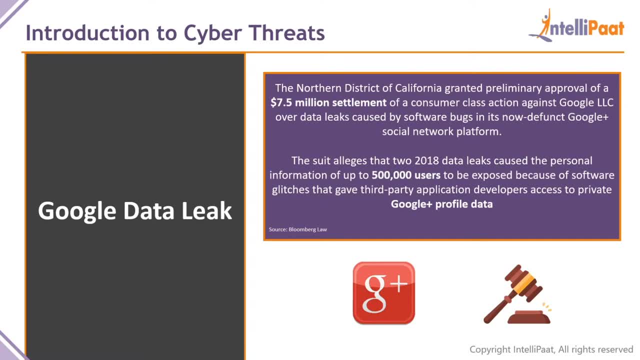 which is known as google plus, if you may remember. so, information of up to 500 000 users was exposed, uh, because of software glitches that gave third-party applications, uh, which you link with google without even looking these days, the access to that data. so, at the end of it, google had to pay. 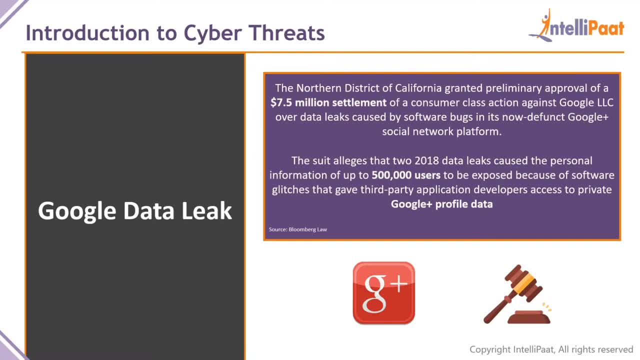 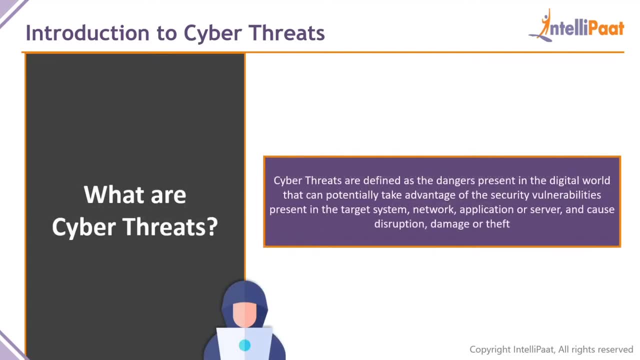 that much sum of money or to basically settle the grievance that the customers had, whose information was essentially leaked. so what is the definition of cyber threats, now that we understand, uh, examples of what cyber attacks and cyber leaks can be all about? cyber threats are defined as the 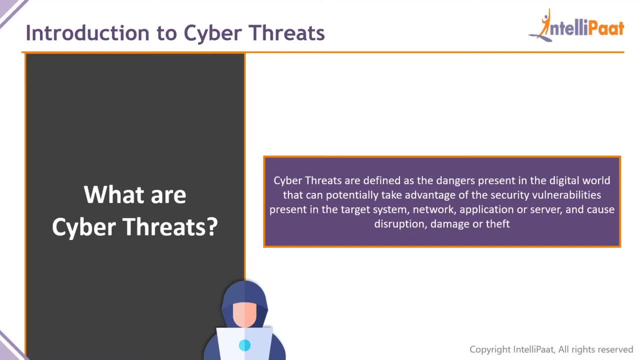 dangers present in the digital world that can potentially take advantage of the security vulnerabilities present in the target system, network, application or server and cause disruption, damage or theft. cyber threats have a very common place in today's digital world. uh, almost every application that you're using, almost every operating system that you're using, has some vulnerabilities, right so? 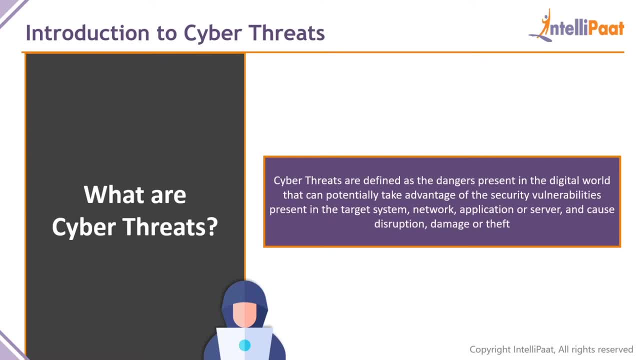 if you're not aware of these things, if you don't operate safely online, if you don't use the proper security measures, if you don't use the proper firewall, the antivirus that you need, you are very, very susceptible to these cyber threats. right, because they are endless in nature. they are always being created on a daily basis. the antivirus databases are: 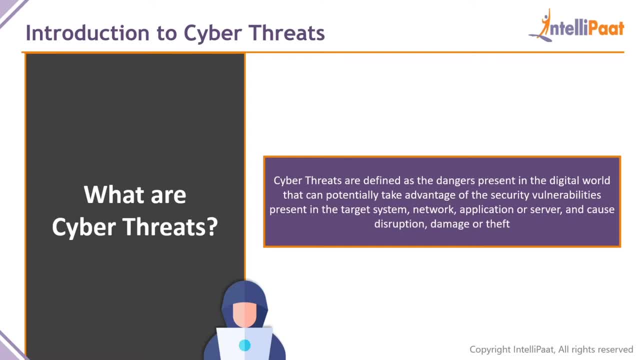 updating on a daily basis based on the new, new sorts of threats that are appearing in the market that can affect your systems. so let us now see how negatively these cyber threats can affect us if we are not careful about them. so, firstly, the effect of cyber attacks. 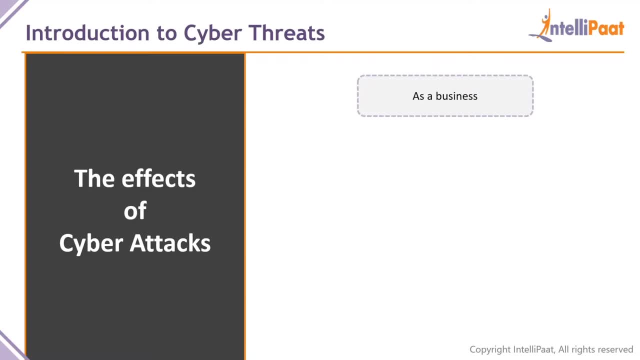 firstly we have as a business. if you're running a business and, uh, you're a victim to a cyber attack, these are the possible liabilities that you can face. so, firstly, litigation- uh, most of all because you're protecting somebody's private data or you're working for an organization that has some 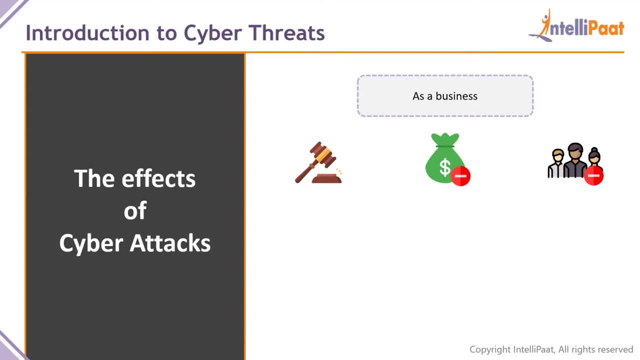 privileged data right and you need to protect that in your databases, in your server, wherever you're protecting it. if somebody gets access to that data, uh, the uh, the suing party, the party whose information has been leaked uh can sue you essentially for the uh damages that they have faced uh because of that right. it could be uh in monetary. 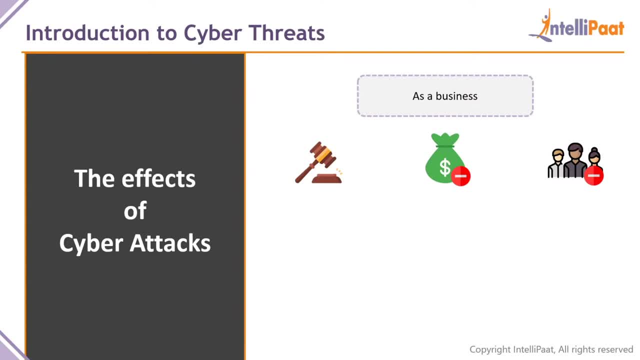 value. it could be in reputation as well, and if it's in reputation, you lose your customer base or your clientele because of it. so, as a business, if you're not careful about cyber threats, you can face litigation, monetary losses because of those litigations and monetary losses because of your. 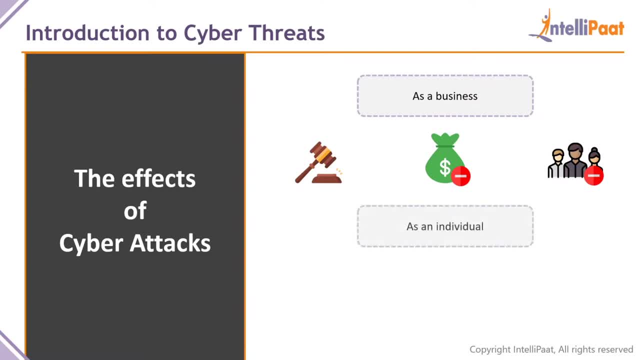 clientele leaving you- and on a personal basis, as an individual, uh, your privacy could be compromised. so that means, if you're using social media and you're sharing some private messages, some privileged conversations, right, your data could be compromised and that could cause you some harm. and, other than that, if you're 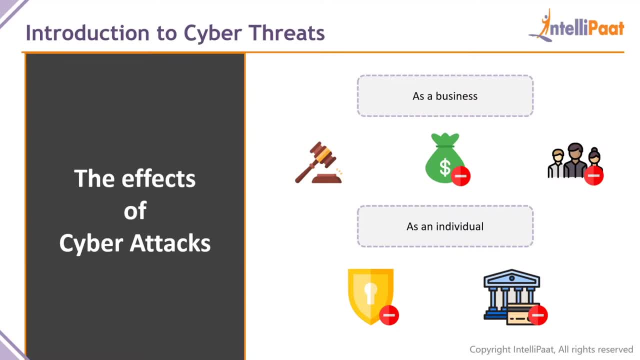 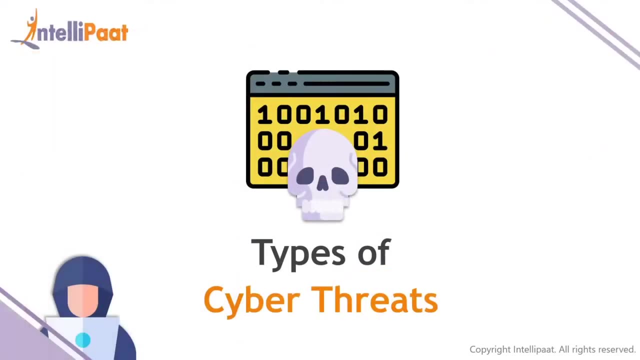 frequently using uh bank accounts online. if your information is leaked, if your session is hijacked, then what could happen is you could lose all your money as well. so these could be the negative impacts of cyber attacks on your day-to-day life. so let us look at the psy. so let us look at the types of cyber threats that exist out there. 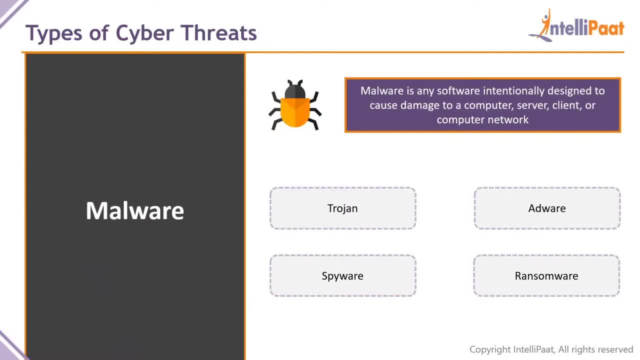 so firstly, let us look at malware now. this i'm sure a lot of you guys have heard about. so theoretically, malware is defined as any software intentionally designed to cause damage to a computer server client or a computer network. the most common uh types of malware are trojan. 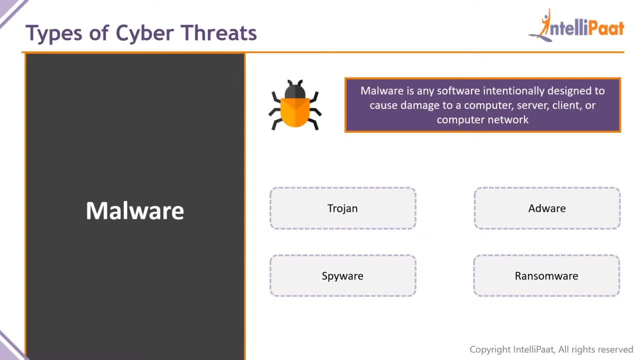 now, trojan is something that pretends to be like an innocent file, right, but it is actually a virus that is present on your computer. so if you, by any chance, try to execute it, what will happen is some negative things can start happening with your computer. some files can start multiplying. 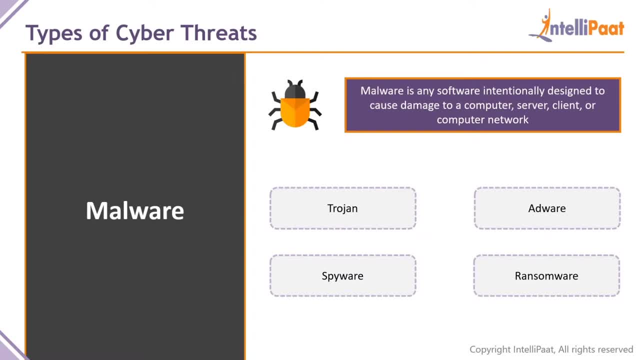 some files can start deleting themselves automatically. your folders could get encrypted. so, essentially, anything that pretends to be like an innocent file but actually turns out to be a malware is what trojan is. trojans are hard to detect, so if your antivirus database is not, 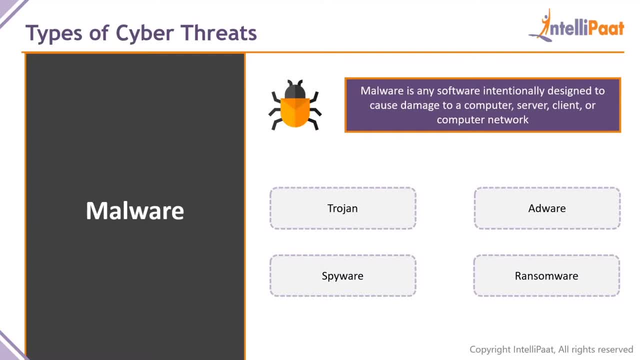 up to date. you're very susceptible to trojans. adwares, on the other hand, are not as malicious as other malwares. so adware essentially is something like that installs on top of your web browser, that installs on your operating system and basically promotes a software that. 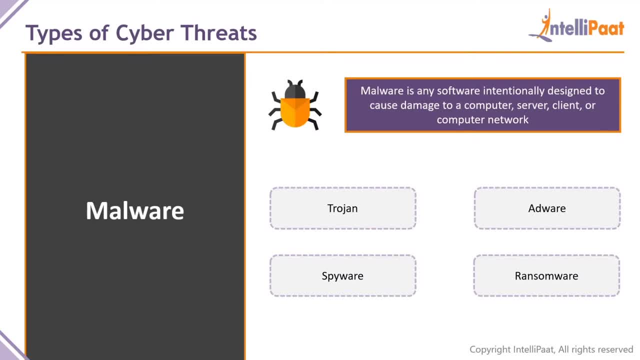 you don't necessarily need, if we were to call it so. adwares are usually installed when you're tricked into downloading a software that you think is from for some other purpose, but you're actually downloading a software that is for some other purpose. these usually happen when there is some negligence, when you're 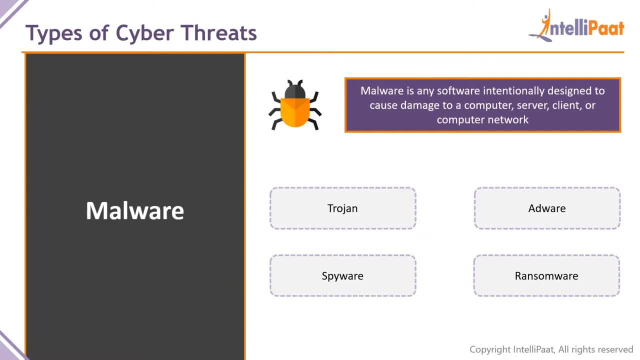 installing something, and you forgot to uncheck a tick mark which says it's it is going to install this particular software. so that is what adware is. and then we have spyware. now, spyware is a more dangerous sort of malware. so what this does is that it installs on top of the operating system. 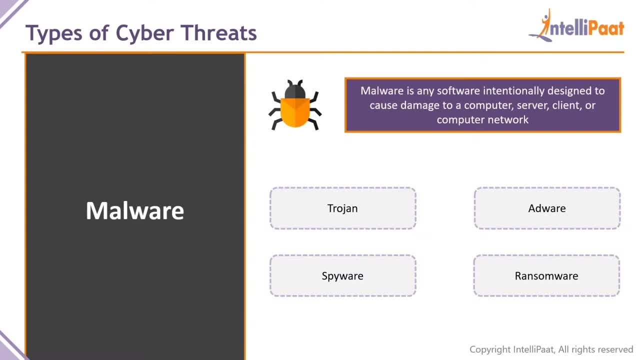 that the target is using now. this could be in the form of a key logger, which means that it is logging every keystroke that you're entering on your keyboard and is sending back that information to the attacker, or it could be recording through your webcam. it could be logging all your web. 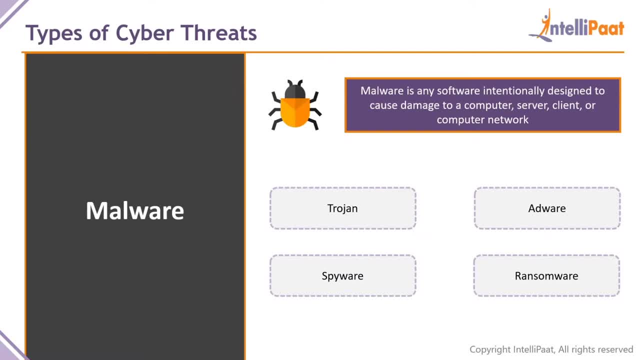 information, whatever your website, you're going on and whatnot. so this is what a spyware is. and then, finally, we have a more recent virus, so to speak, which is called the ransomware. now, ransomware is something that if you, if it is installed on top of your system, 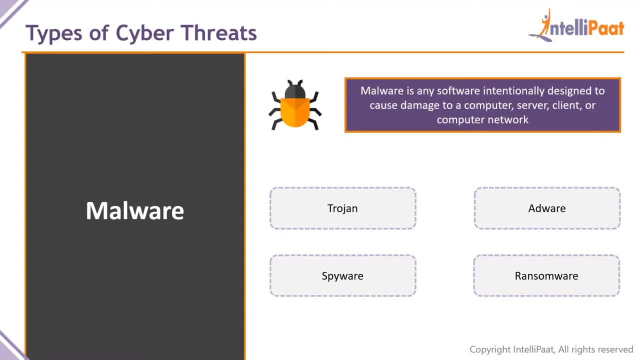 it'll. it'll essentially encrypt your file system right and encrypt all of your data with a password, with a passphrase, so to speak, and then, after the encryption has happened, you'll get a message on your screen that if you want your data to be decrypted and you want the 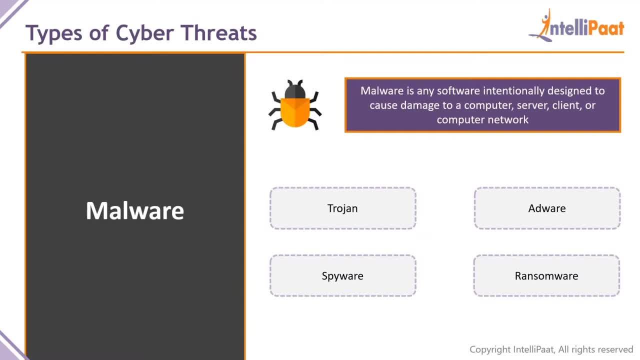 key phrase to decrypt it. kindly send x amount of money to this bitcoin wallet or x amount of money to this particular bank account. so usually bitcoin wallets are used because they are untraceable in nature. these sort of attackers do not use their actual bank accounts, so until you send them that, 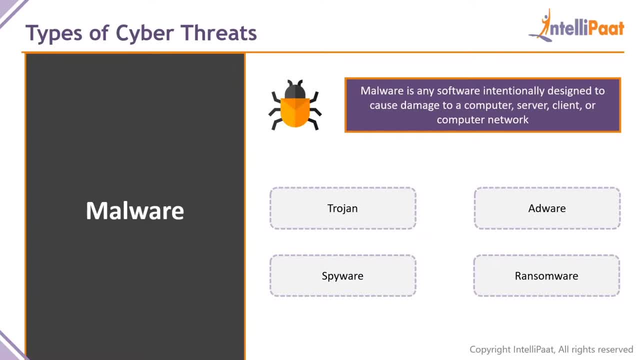 money, you will not have access to your files present in your system and even if you send them that money, you still have no guarantee whether you will get your access or not. so you can see the severity of these threats that can happen. so they could range from normal. 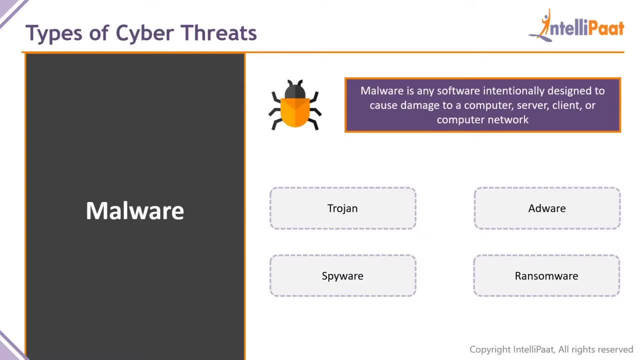 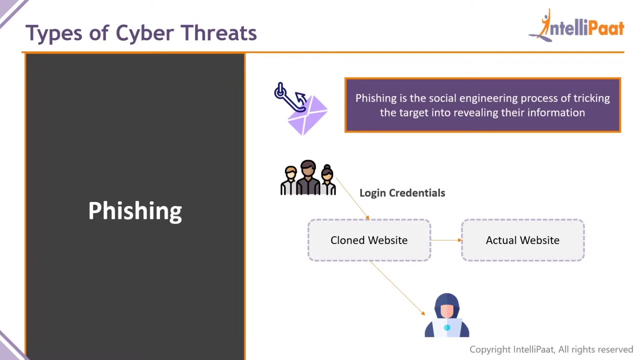 annoyances like adware, to these superior viruses like spyware and ransomware, which could- which could potentially- cause you a lot of harm as well. then we have phishing. phishing is something that can cause you a lot of harm as well, although it is not that prevalent today. 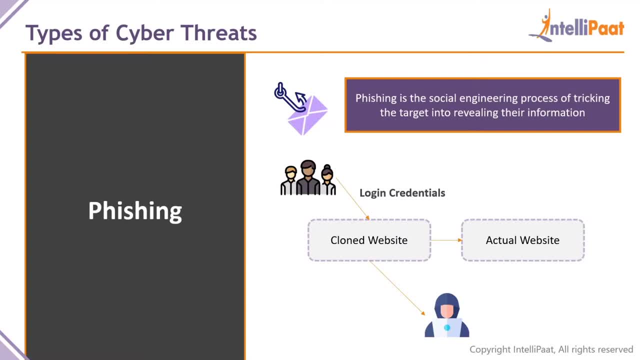 but it's still a very common thread that exists out there for websites with low security factors. so, for instance, phishing is the social engineering process of tricking the target into revealing their information. so, for instance, you create a clone of facebook, so facebookcom is the actual website. you create something like facebookxyz. you send that link to. 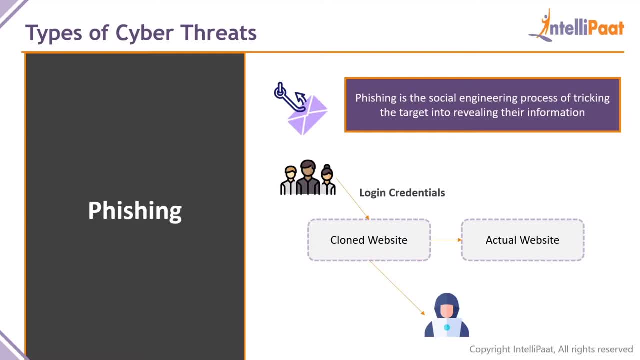 your potential victim. so when the potential victim sees that facebookxyz link, he clicks on it. he gets access to a website that looks identical to facebook. so if the person is not fully aware of what he's doing, he might enter his actual login credentials and the login fields of that particular cloned website. so what will happen then? 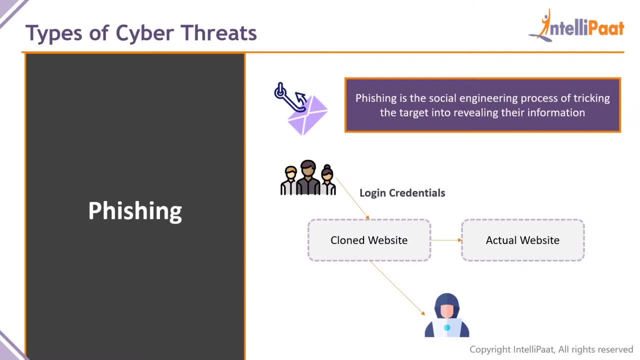 In that case, what will happen is you will get access to his email account and his password in plain text format. so that means you will get access to the email and password in the default format details afterます, without any encryption right. and then, if you're smart enough, what your cloned website will do is 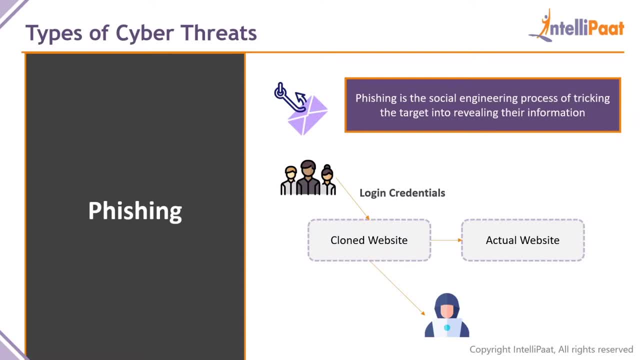 that it will actually redirect this individual to the actual website so that the person does not suspect anything. so he, the person, will log into facebookxyz and he'll log into his original account and he'll not suspect anything. but you'll have access from then on to his email id and 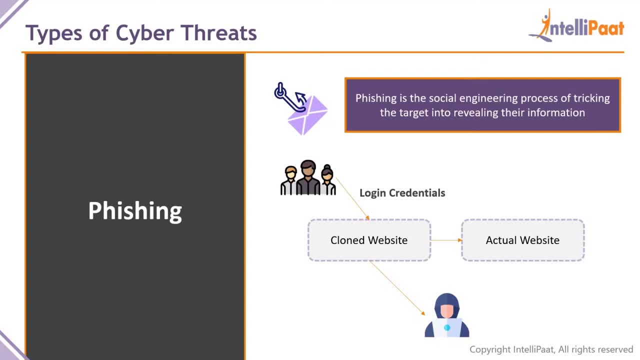 password. so if you want to log into that facebook account anytime, you can do that as well. so this is what phishing is. it essentially depends on the person being dumb enough to basically be fooled by a cloned website by not checking what the website is and what the name of the website, the url of the website, is. 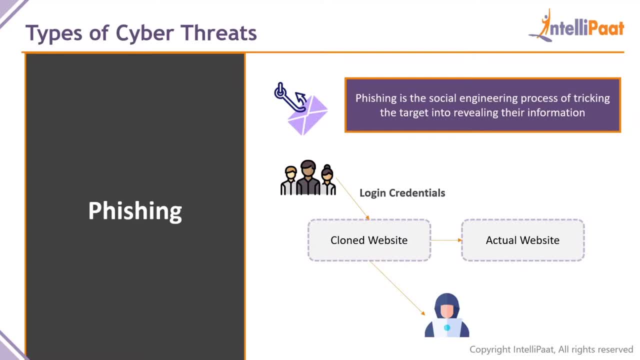 this is also very preventable these days with the use of two-factor authentication where, even if you enter the password correctly, it will still send an otp to your mobile phone. so until you enter that otp, you still cannot have access to the account that you're trying to get into. 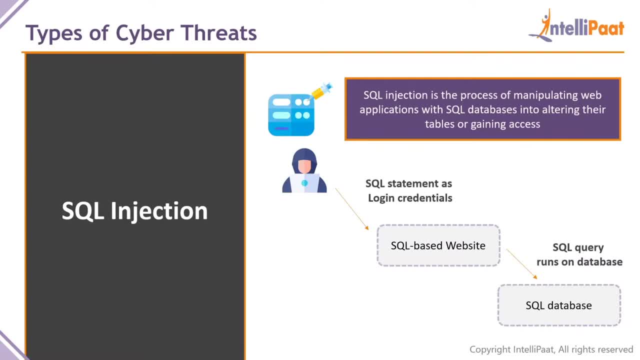 next up, we have sql injection. now this is also easily preventable. so what happens in this particular attack is that the attacker will enter an sql statement in the login fields, so say, for instance, if a website is using an sql database. so what the attacker will do. 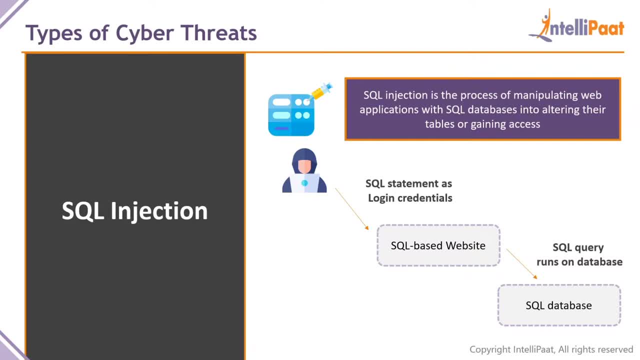 is that that attacker will enter instead of the email id. the attacker will enter a intelligently crafted sql statement so when, on the server's back end, that particular entry field is compared to the actual emails that are present in the sql table, the way the statement has been crafted, what it would prompt that database to do. 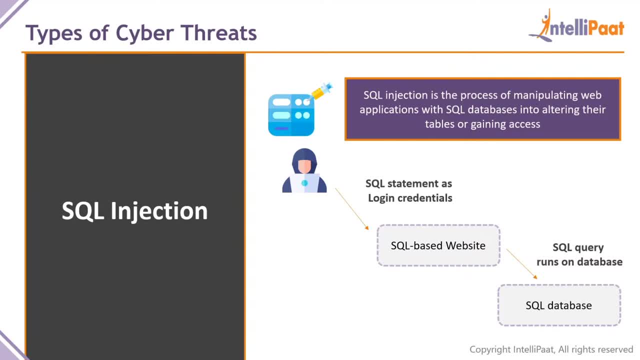 is some other activity as well, so essentially you're running a query on the target website's database, so you can essentially do anything with it. you can alter the table. you can add new records to the table, which means you can add your own record to the table. you can create your own account without 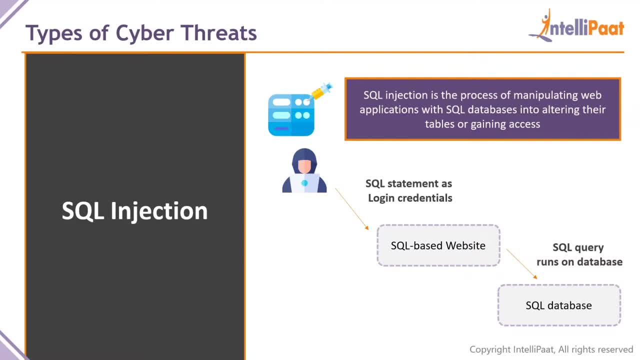 actually creating it right, and you can drop tables as well. you can drop entire databases as well, right? so this is what sql injection is. there are security measures that are put into place for sql injection attacks. for instance, instead of actually running these- uh, these entries on the database itself, you can simply bring the data from your database and then do it on the. 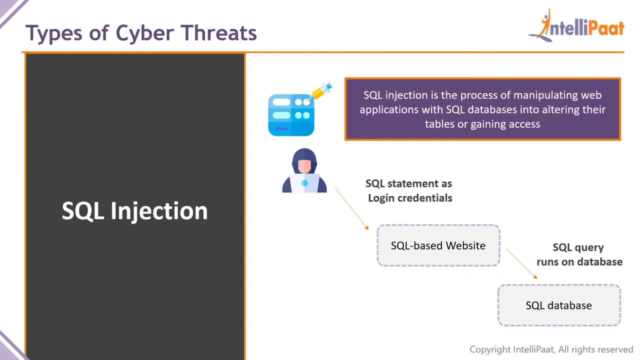 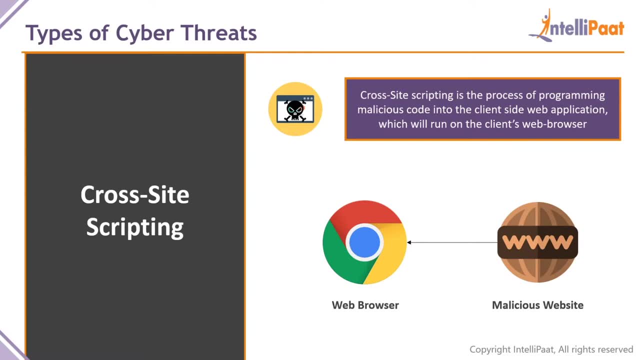 server's end instead of the database end to prevent these sorts of attacks. cross-site scripting. now, this is also one of the most common sorts of cyber threats that exist, and you must have encountered it as well. so on good websites, on authentic websites, this does not happen, but if you're 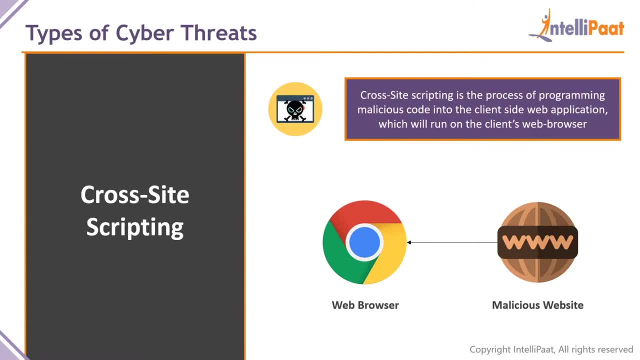 going into some shady website, right? so what will happen is: uh, there, every website, essentially uh- will send some javascript code onto your web browser for execution if it has dynamic elements to it. so within those javascript code blocks, if somebody embeds some malicious code, right, that would also run on your web browser in order to render that. 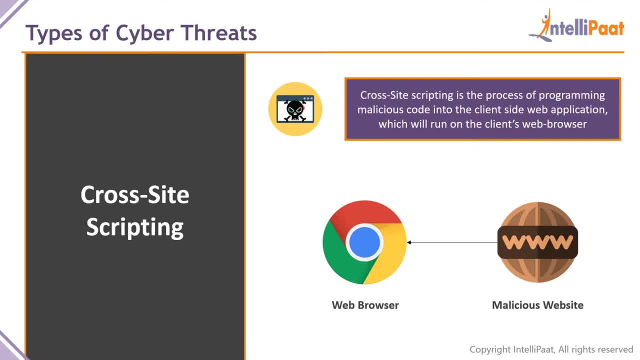 website or to basically execute the functionality, the dynamic functionality of that website. so if your browser security is not good enough, what could happen is you could run some script on your web browser that could cause a potential harm to your system. it might install some sort of a backdoor to your particular web browser where the attacker can have access. 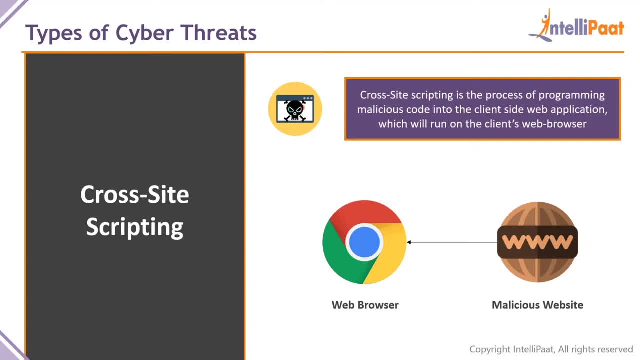 to the information of whatever you're visiting or whatever you're typing on the web browser. so this is what cross-site scripting is. so never click on links that you don't know about. never go to websites that are not secure. don't click on a random download links, right? so that is the reason. 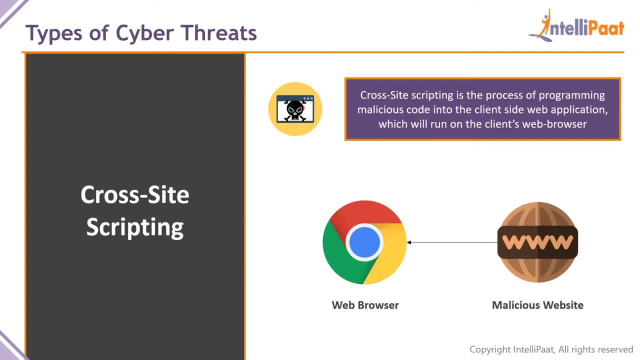 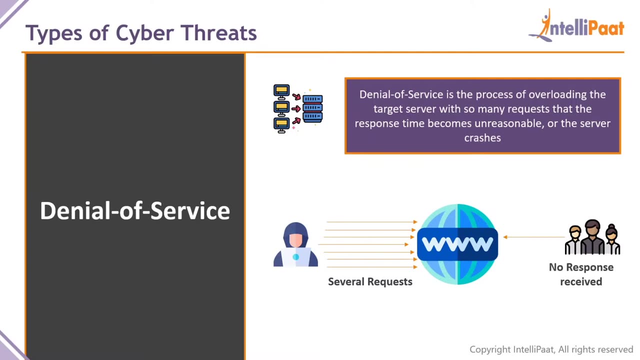 your browser could get infected with cross-site scripting. it could also install adware onto your web browser or could, or it could do a much worse activity as well on your web browser. then there is denial of service. now denial of service is the process of overloading the target server with so many requests that the response time becomes. 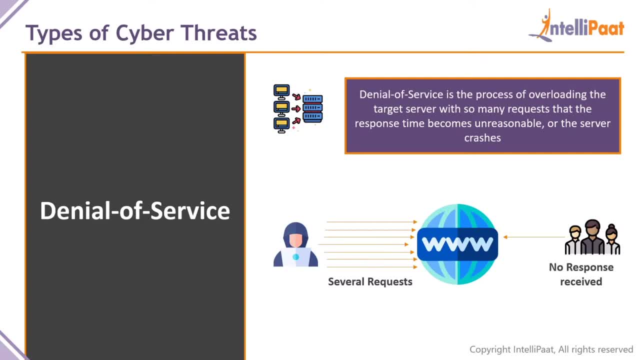 unreasonable or the server crashes. so basically, in this attack, what happens is the attacker will send thousands and thousands of requests to a web page or a web server and, once those requests have been sent, if the server does not have the appropriate resources to deal with those many, 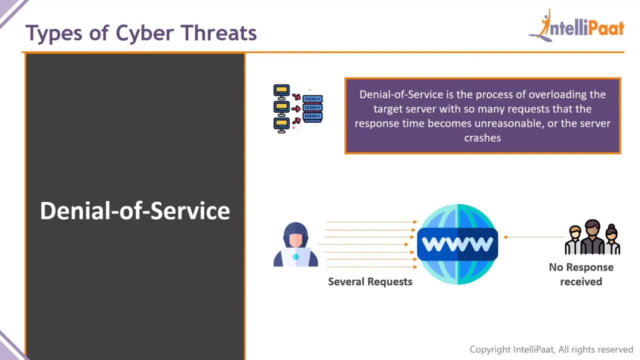 requests, the server overloads. and when the server overloads it becomes extremely slow or it crashes and because of that no other user who's trying to access that website or server can access it, essentially denying them that service. and this sort of attack is called denial of service. 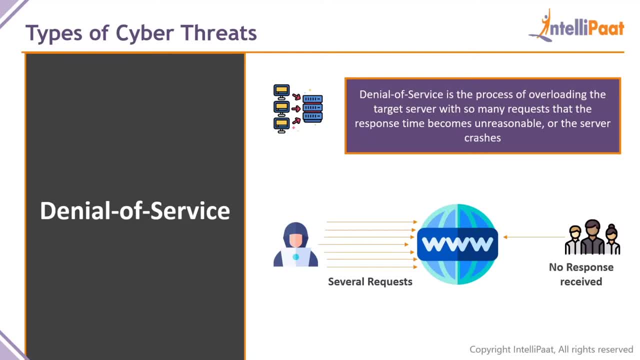 there are a lot of counter measures to it. you can ip block that particular attacker, right. if the attacker is attacking from multiple ips, there are other counter measures for that as well. one of the counter measures is using some a service log like cloudflare, right? so this is what the denial of 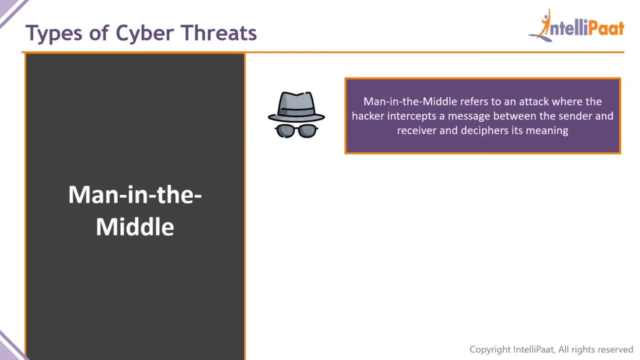 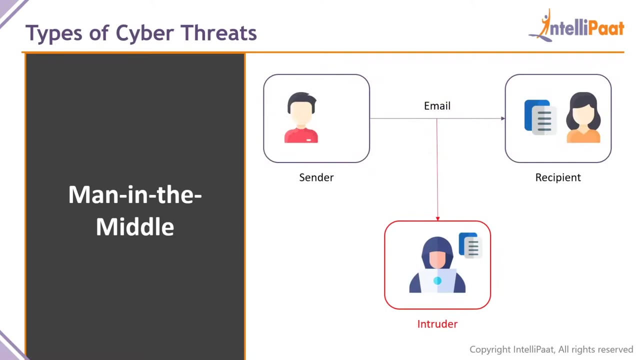 service is, and finally, we have man in the middle. so man in the middle refers to an attack where the hacker intercepts a message between the sender and the receiver and decivers its meaning right. so if you are sending a message to a sender, you are sending an email to a recipient. if an intruder